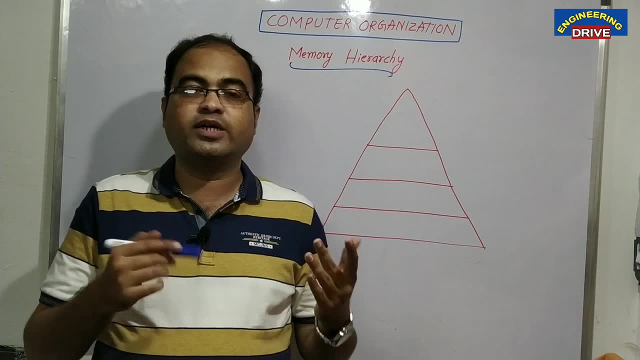 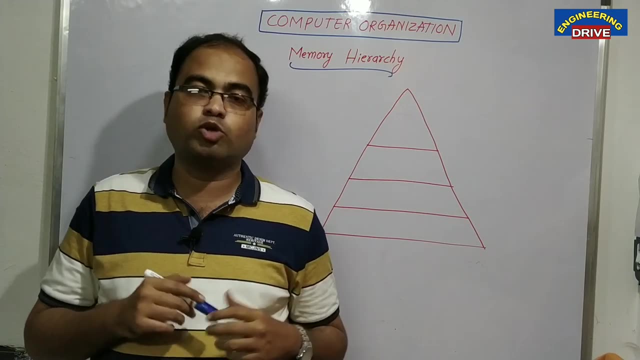 available in a computer that can make together to increase the performance of our computer. So what are the different types of memories and what are the uses of those memories and how they will work collectively that I am going to discuss with you in my today's video. 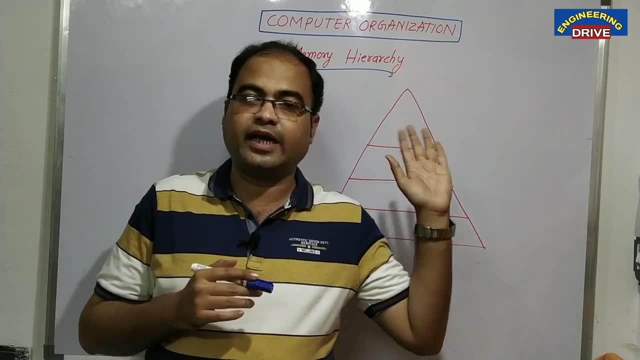 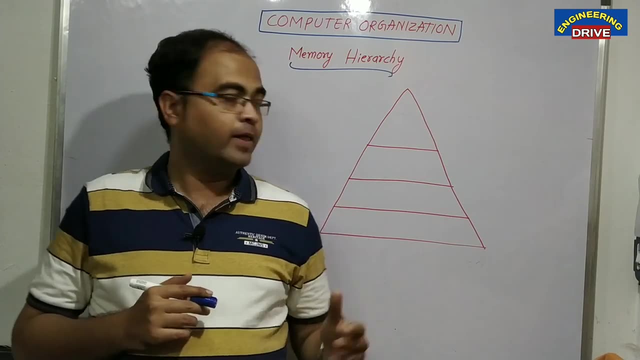 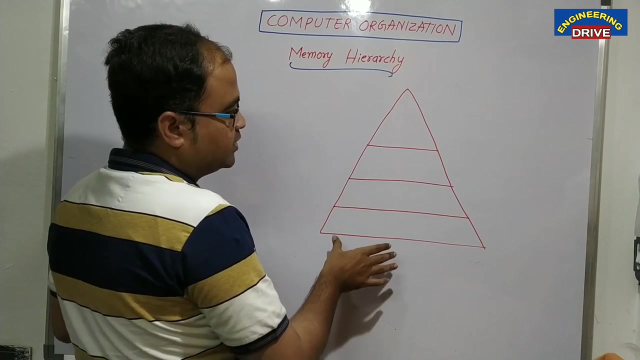 So let us discuss about the hierarchy of memory. What is hierarchy? Whenever I am using the word hierarchy, Levels. hierarchy means levels. Okay, now here in our example, let us say I have drawn one pyramid shape here You can see, here at the bottom you can see, the width is more and when. 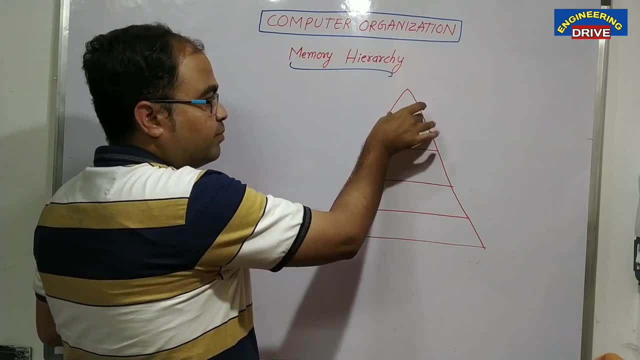 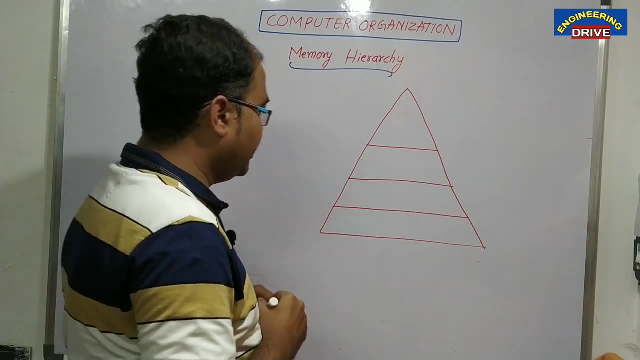 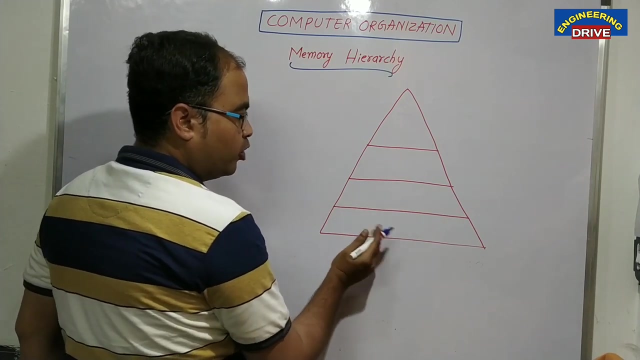 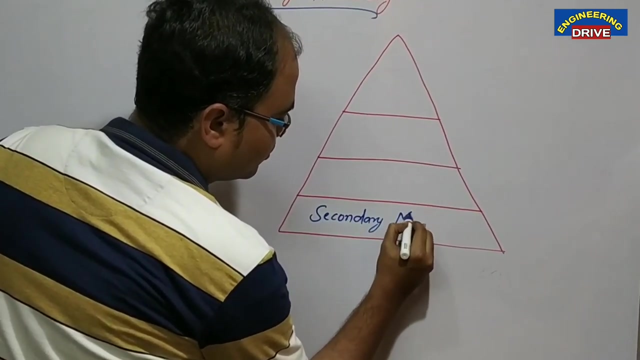 you assume it is. as it is going to the top, the width is becoming less. So what is the difference between that and what is the logic behind the diagram? I'll be telling you. okay, see here the bottom most part of our memory In our computer. the bottom most part of the memory is our secondary memory. 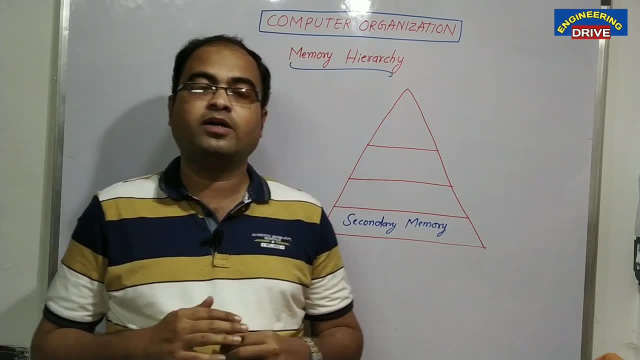 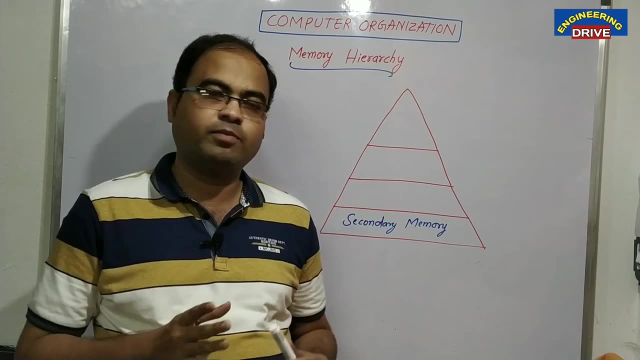 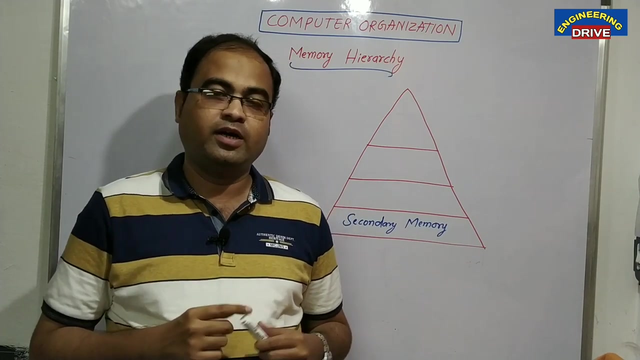 You know what is secondary memory. Secondary memory is nothing but our external memory. That can be our hard disk, that can be our pen drives or that can be our CDs or DVDs. They are all comes under the category of secondary memory. Every computer will have secondary memories to store large amount of data. 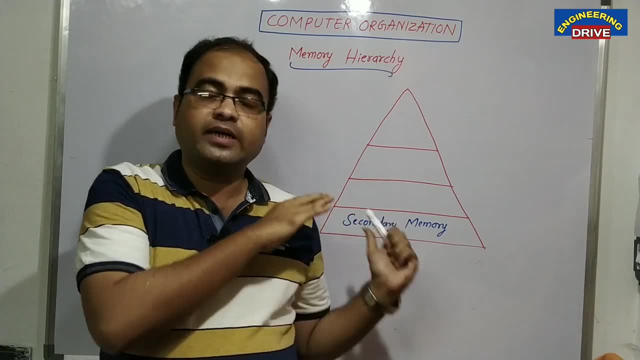 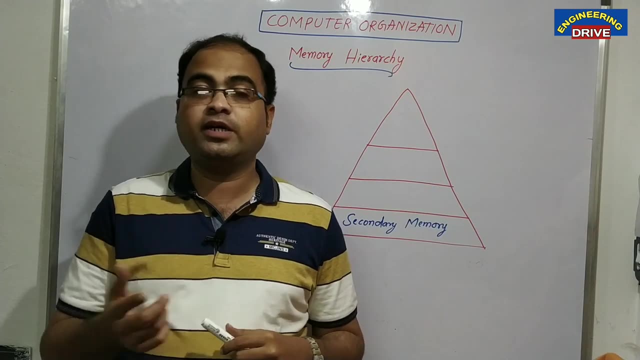 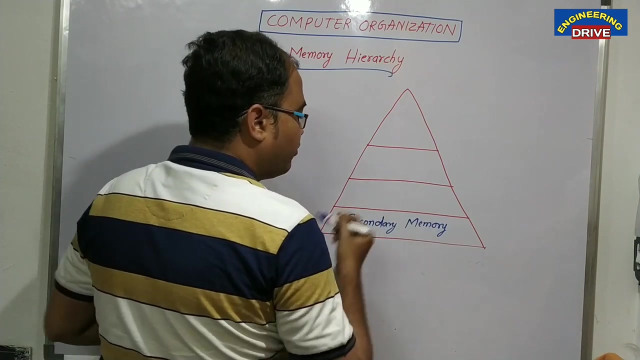 And why I have written this secondary memory at the last? because secondary memory sizes are very, very large. They can store enormous amount of data in terms of gigabytes or even in terabytes also. Okay, that's why I have written secondary memory Once. after this layer, our computer will make use of one very, very important memory: that 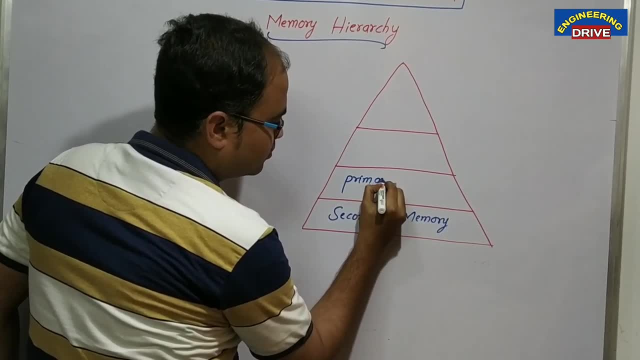 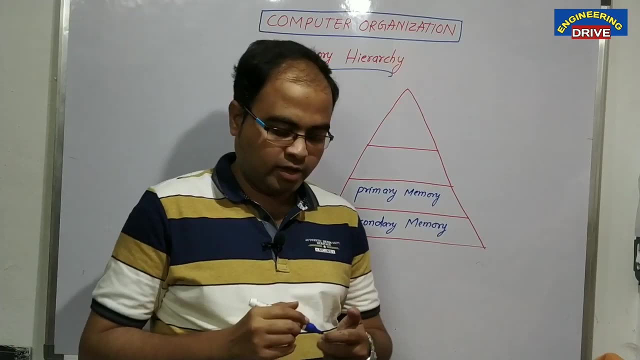 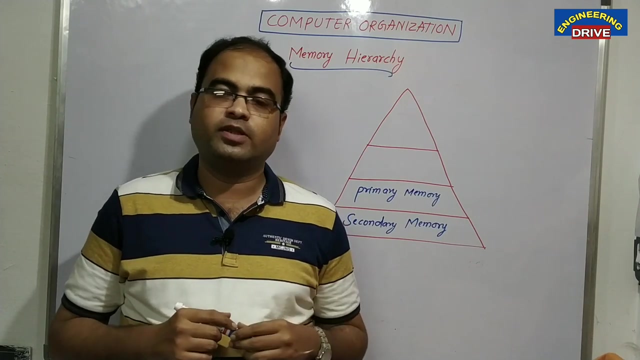 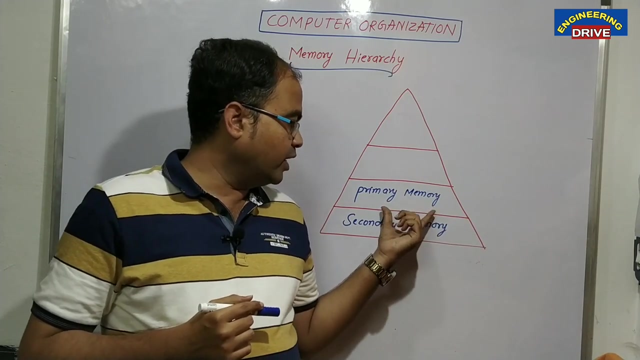 is our primary memory. Okay, what is primary memory? Primary memory is also known as main memory. Primary memory example is our RAM and ROM. They are all examples of primary memories because without RAM there is no use of our computer also, So primary memory- the size of primary memory- is lesser than secondary memory, but it is 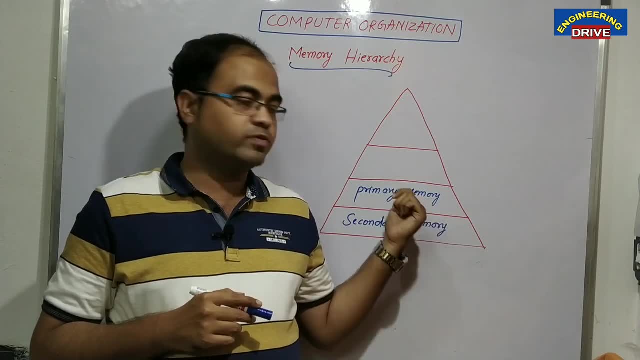 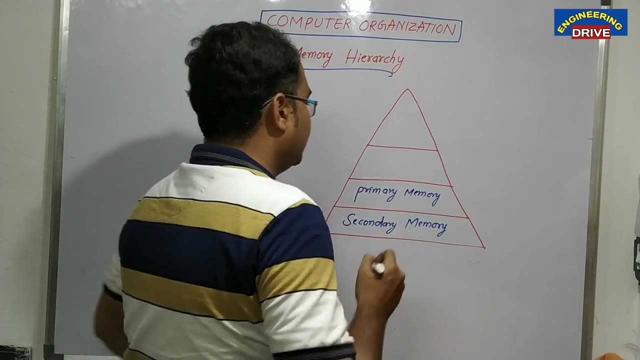 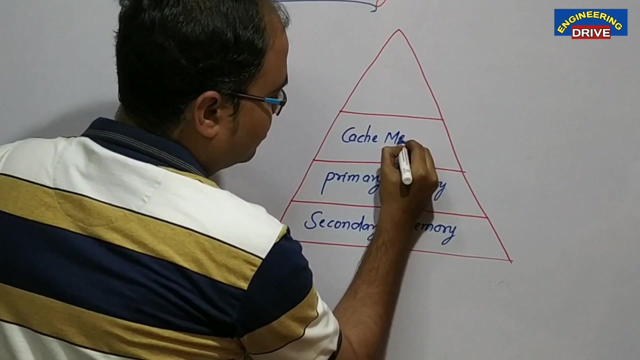 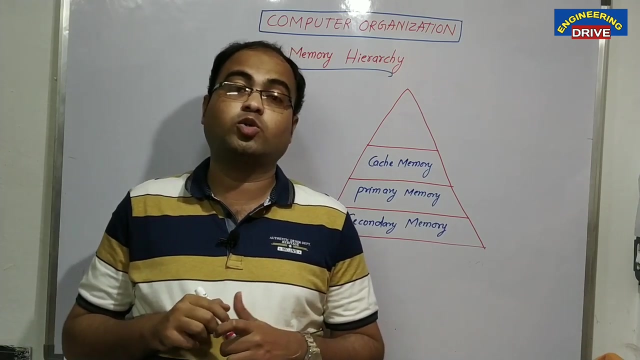 a very, very important part of our computer, because without primary memory our computer won't work also. So the second layer- I am going to add primary memory- and then the third important layer of our memory hierarchy is the cached memory. Now our computer will make use of cached memory also in order to do work much more faster. 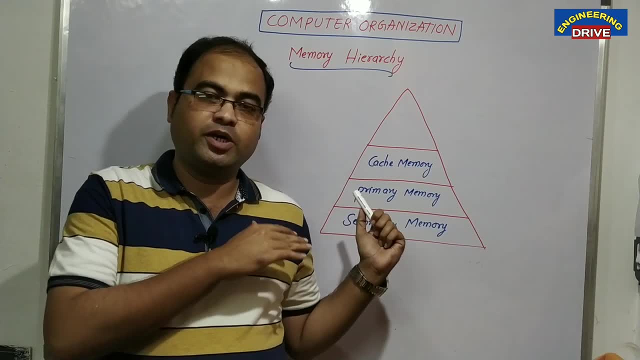 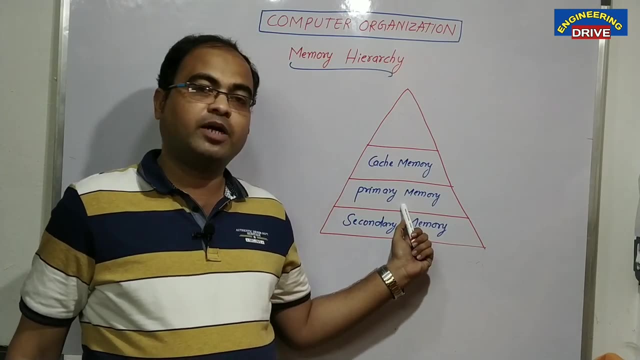 Okay, what are the uses of all these memories? I will be speaking you, I will be telling you once. I will complete this diagram. So the bottom, most layer, is secondary memory, Then computer makes use of primary memory, then cached memory and the smallest layer. 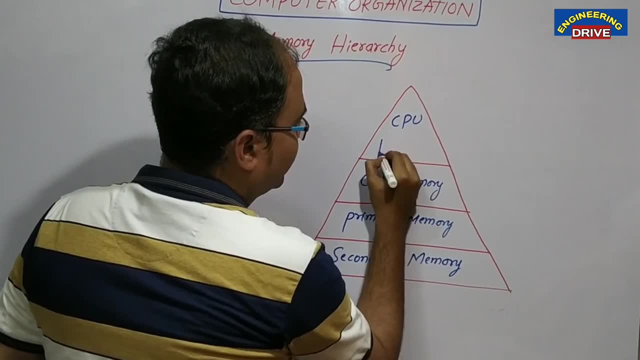 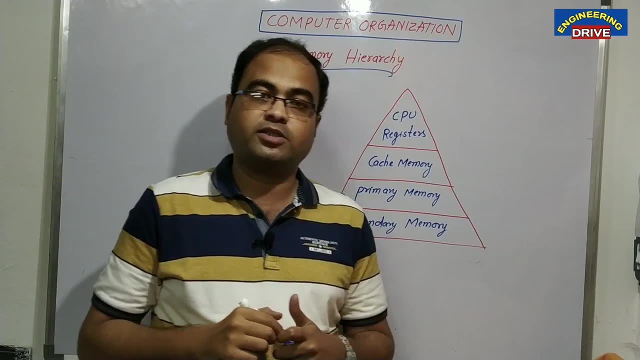 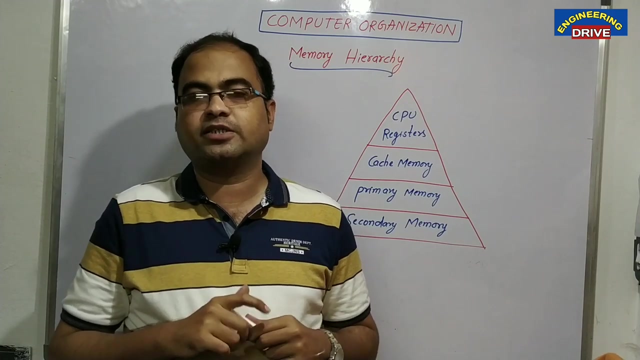 is our CPU registers. As you know that in our CPU also we are having three important parts. One is ALU, CU and registers, arithmetic and logic unit, control unit and registers. And registers are also very small components in which data can be stored. 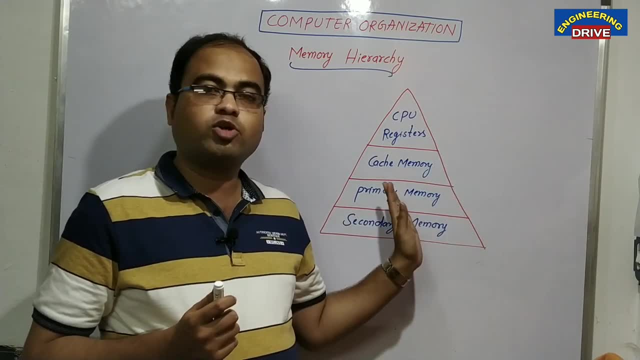 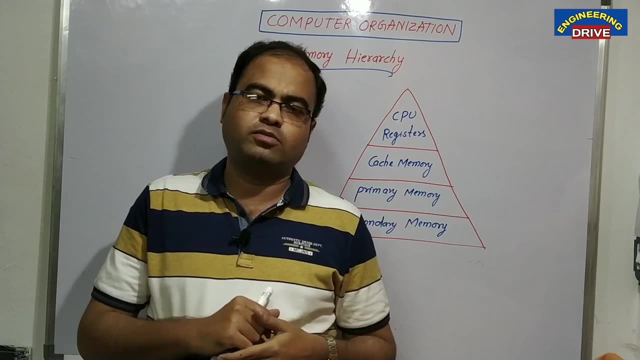 Okay, Our computer will make use of these four types of memories to produce the performance. Now the answer is, sir, which one is very large and which one is very small. now, So by seeing the pyramid, you can say, you can say, think that secondary memory is the. 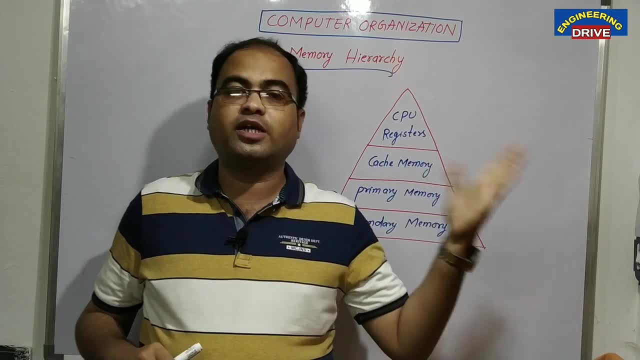 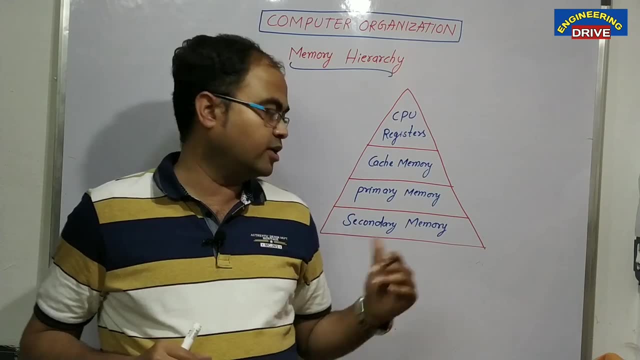 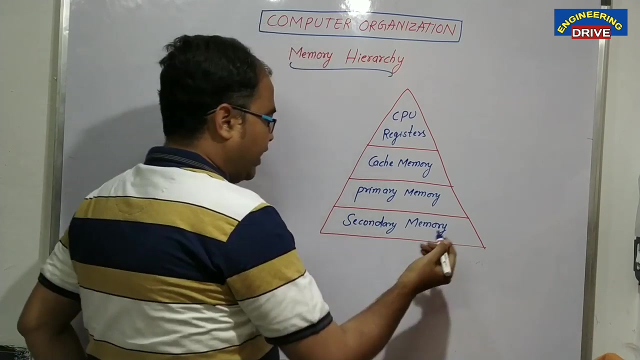 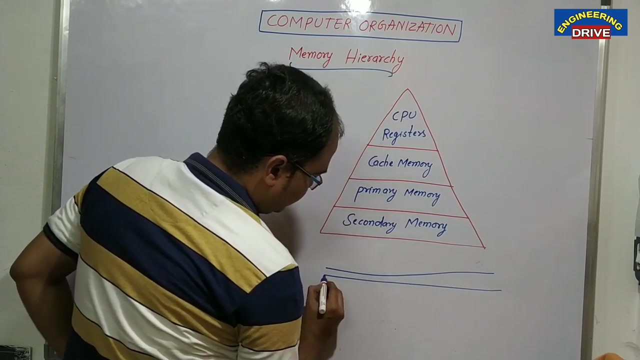 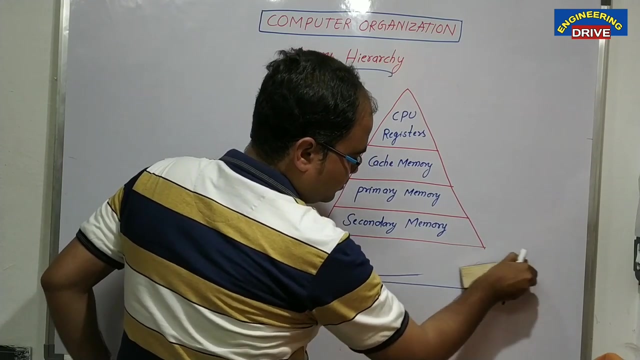 largest memory, whereas CPU registers are the smallest one, which means CPU registers can store only a very small information, small amount of information, whereas secondary memories- they- can store large amount of information Or data. that's why we can keep one arrow here. that is okay. let me erase this one. 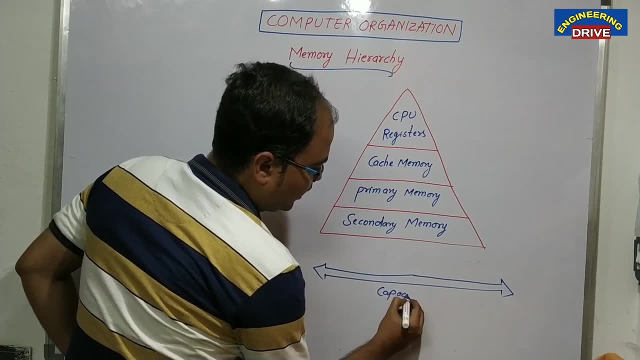 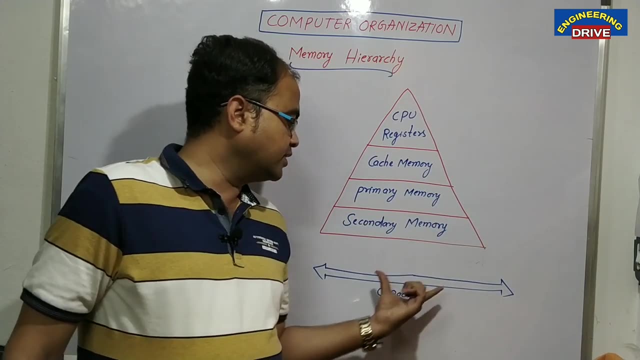 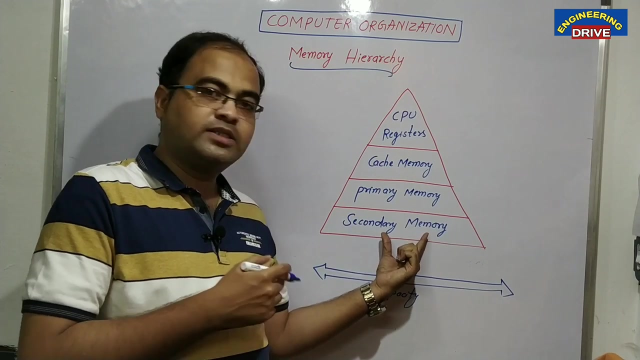 So this is nothing but our capacity. So this broad Line, this broad width indicates of the pyramid that this is the capacity. It, as it is going narrower, it indicates that the memory size is getting smaller, So largest one is secondary memory. 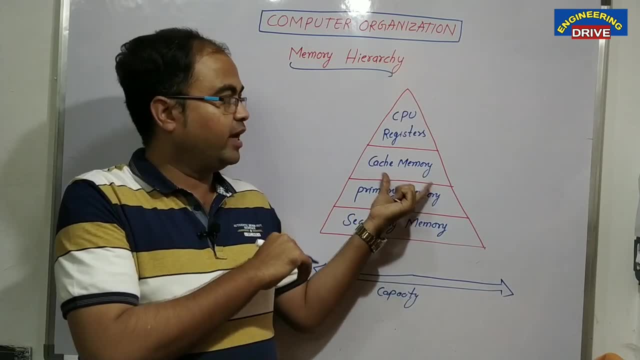 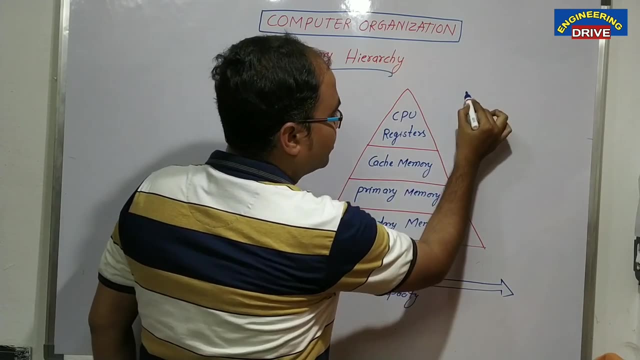 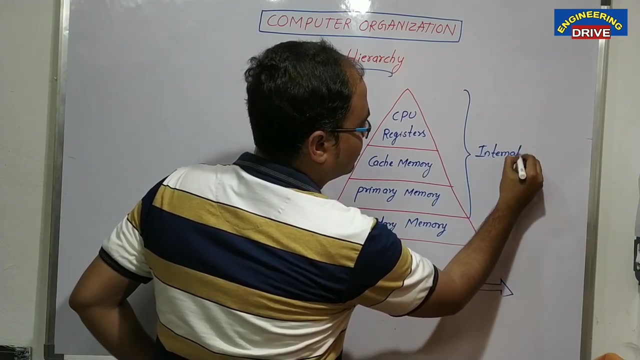 Then comes primary memory, then somewhat smaller cache memory and then most smaller CPU registers. And one more thing is this: CPU registers, cache memory and primary memory, They are collectively formed together as- Okay, Okay, Okay, Okay, We call it as internal memories. 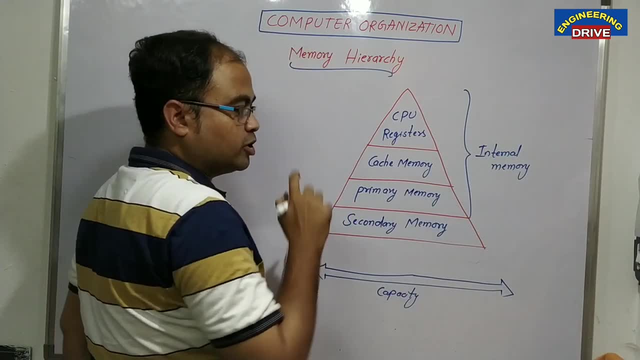 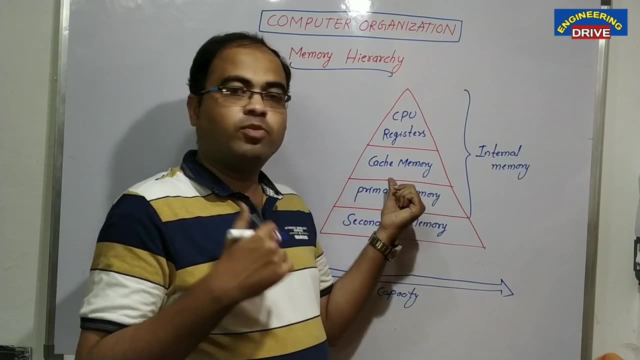 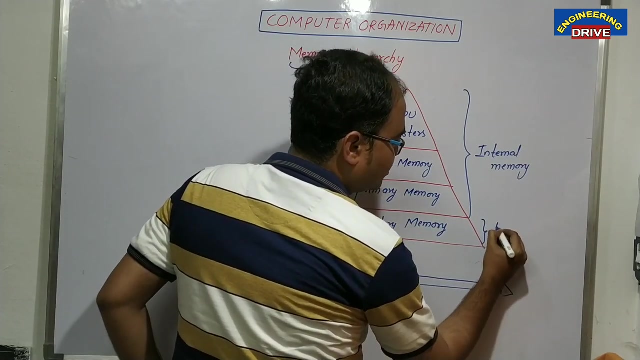 They are called as internal memories because they are available inside the system. That's why these three memories are internal memories. RAM is available inside, cache memory is available inside, as well as CPU registers also available inside, Whereas the secondary memory it is known as what we call the secondary memory. 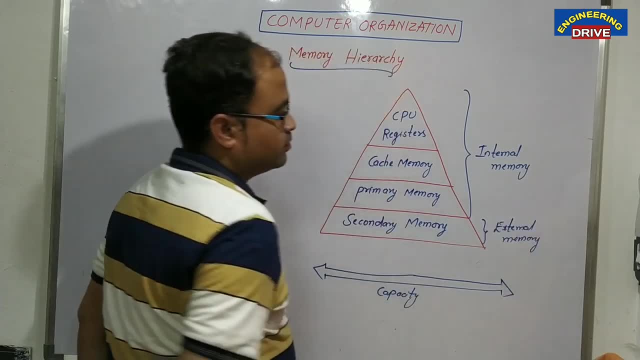 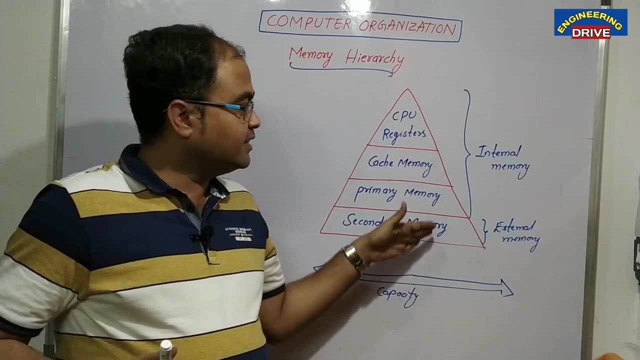 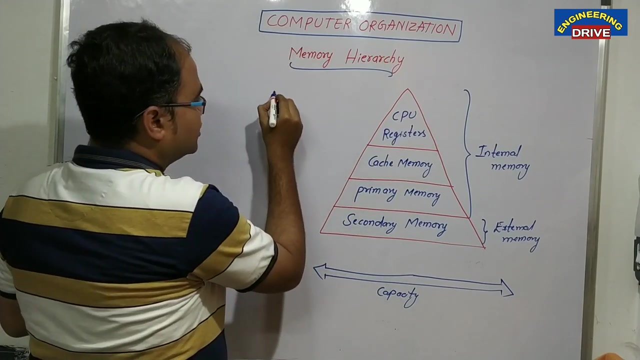 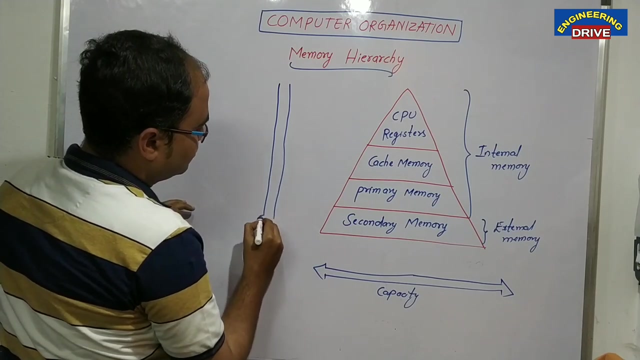 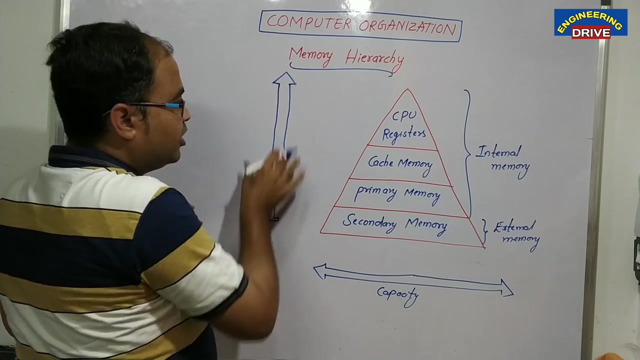 External memory. We call this secondary memory, External memory memory. okay, we can see that from bottom to top, size is getting reduced, yes or no. but if we take in reverse- suppose if i draw arrow like this here- then what is the meaning of that increasing? 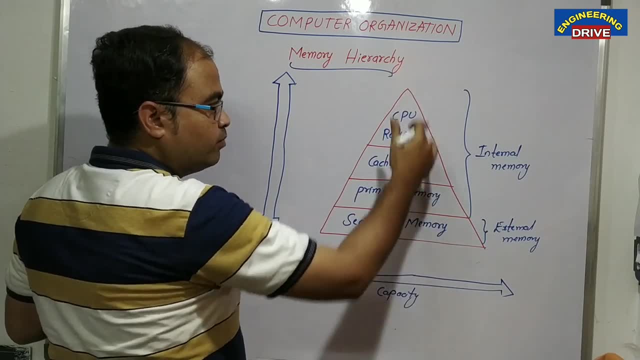 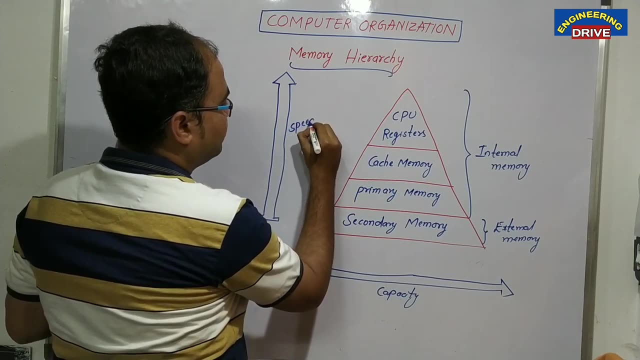 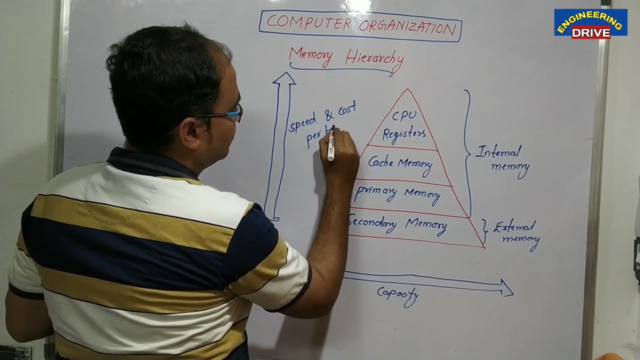 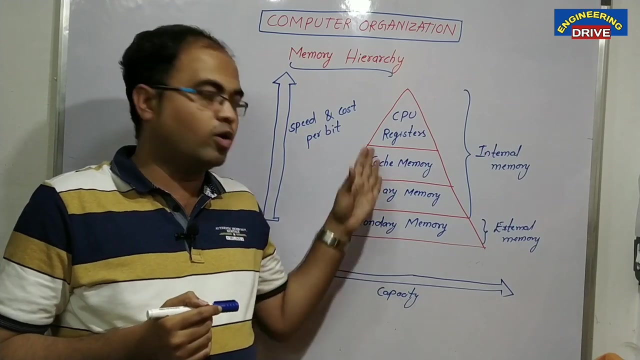 here. in this case, the size is getting increasing from top to bottom, whereas from bottom to top what happened? speed and cost per bit, which means which is the very costly and which is the very fastest memory out of in this, out of this four we can say cpu registers. they are the much more 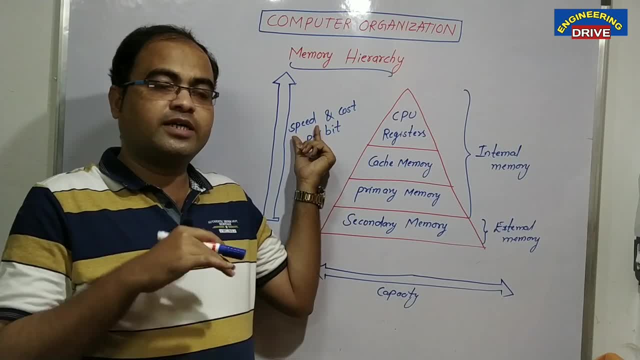 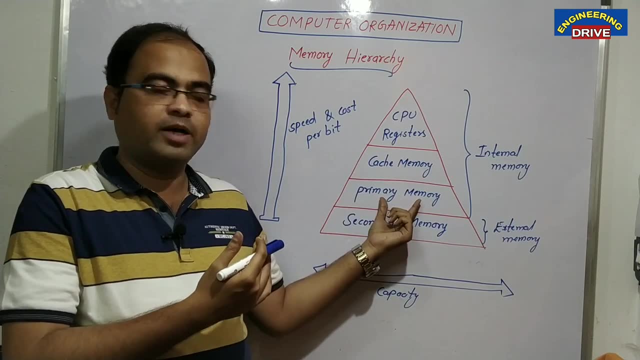 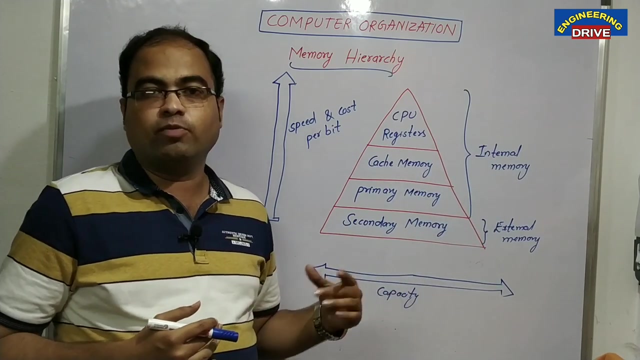 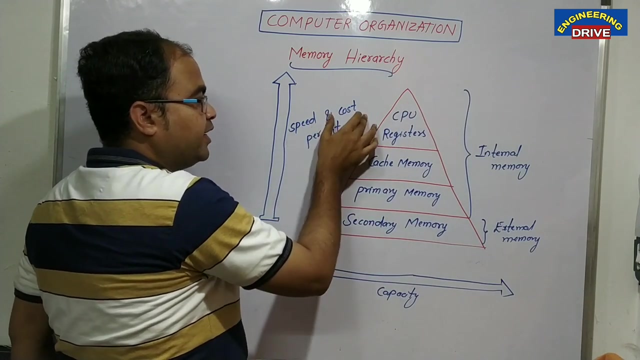 faster ones and speed. another thing is they are very costly. then somewhat cheaper case memory, then somewhat cheaper primary memory and very low price is secondary memory. but in reverse, secondary memory is the largest memory. see here, from bottom to top the size is getting decreased, whereas in terms of speed and cost, from bottom to top- speed as well as cost of the memories.